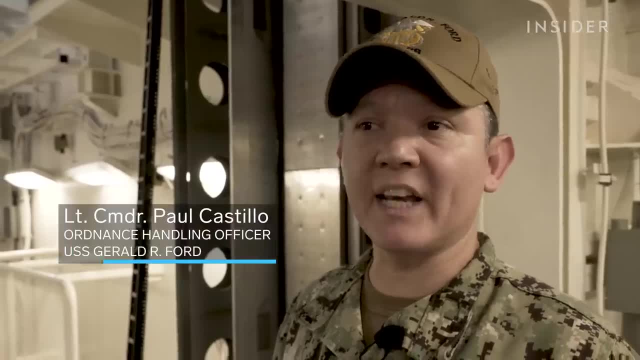 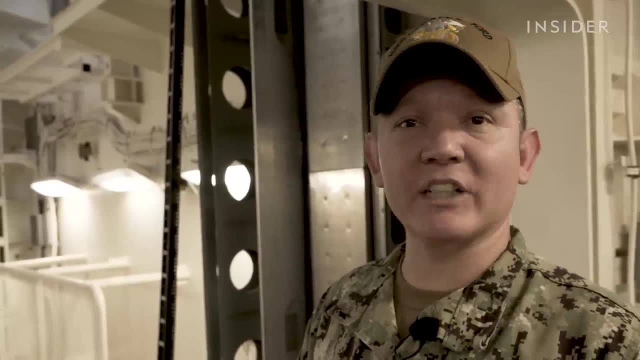 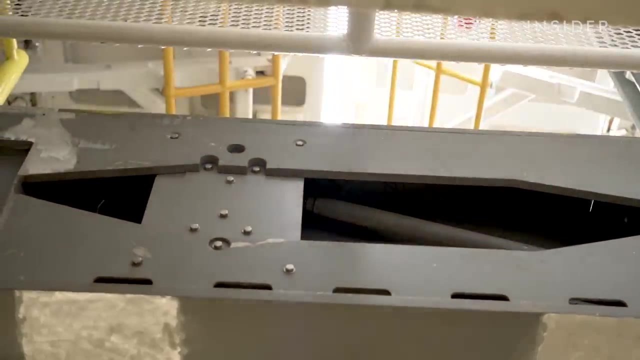 We're bypassing the mess deck area. We're completely independent. You would never even see us move an ordnance throughout the day. So it's more secure with higher survivability and we can store more on board. It's the only way to move munitions from deep inside the Ford to rearm planes on its flight. 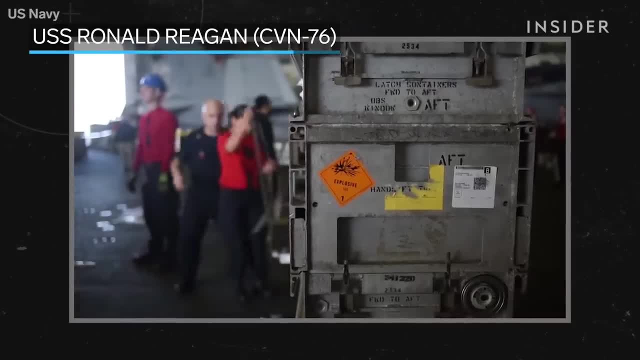 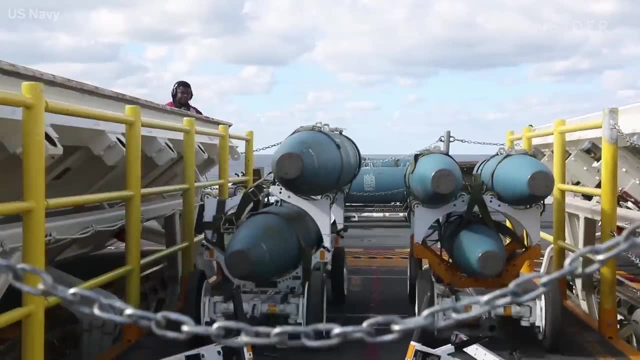 deck. Less advanced carriers move weapons on board. Less advanced carriers move weapons on board. Less advanced carriers move weapons on board. Not only that, They ship their weapons in a more dangerous way from hangars to the flight deck. There are 11 elevators on board, yet only 7 are fully functioning. 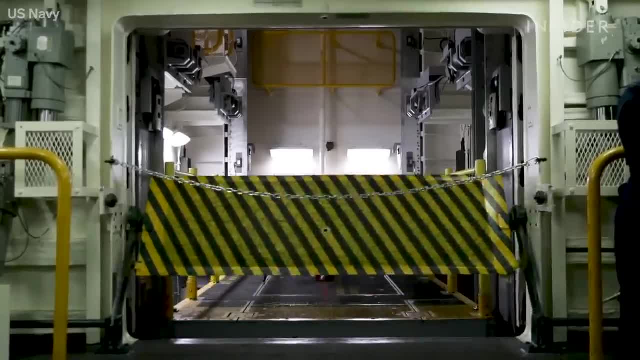 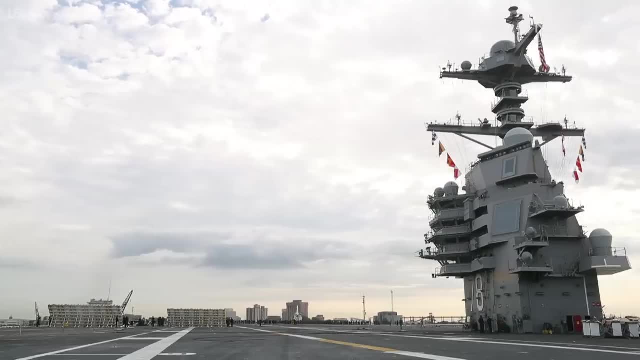 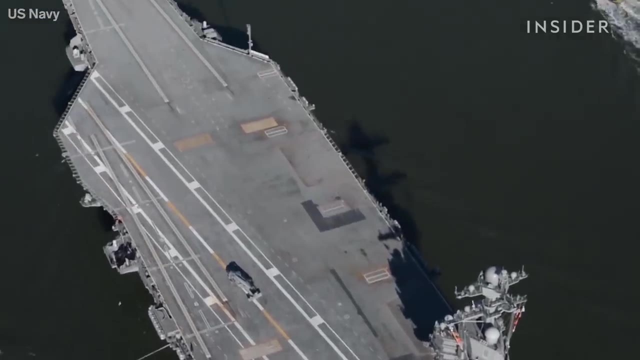 Until all 11 elevators are complete, this ship can't be certified for deployment. The Advanced Weapons Elevators are just one example of nearly two dozen major new technologies that make the USS Ford cutting edge, AND one big floating experiment, Tal Manville, are now include going on a day or two tour. 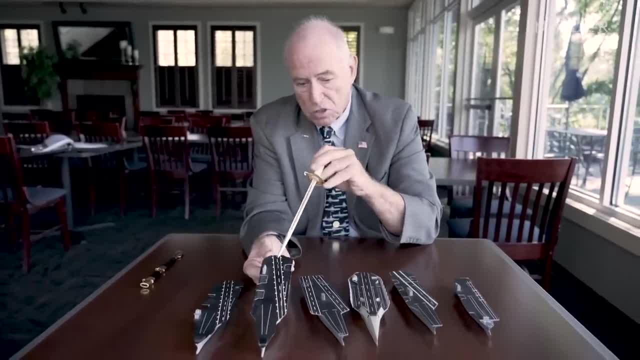 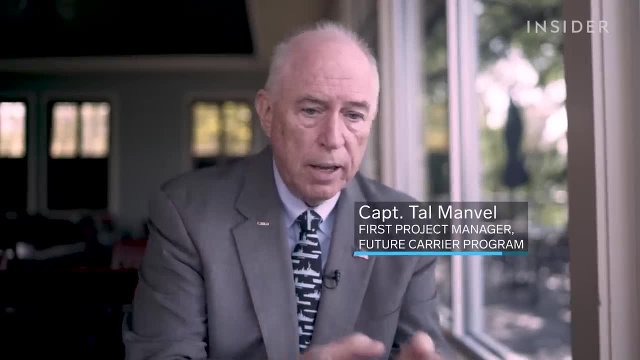 John Voll is a retired Navy captain who served as the very first project manager on this new class of aircraft carrier. The ship was supposed to start construction in 04.. It got moved to 05.. They made an adjustment. They delayed it a second time. They delayed it a third time, Pushing that out. the ship, just by those delays, went from $6.4 billion to $10 billion. The Ford is the first of four new carriers already in different stages of design and build. The Navy plans to replace the entire supercarrier fleet with Fords. 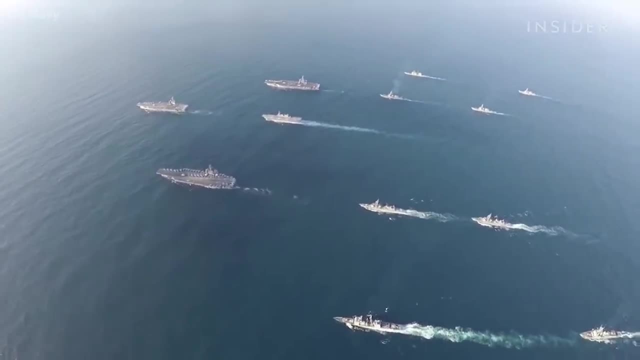 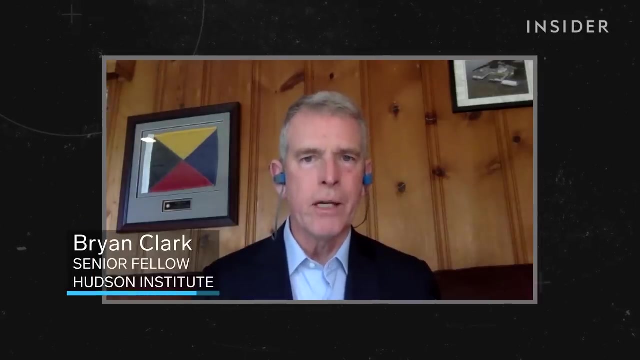 US law requires its Navy to operate 11 carriers at all times, But with all the delays the US is down to 10.. The reason we have 11 is driven by the fact that the US Navy is kind of a two-ocean. 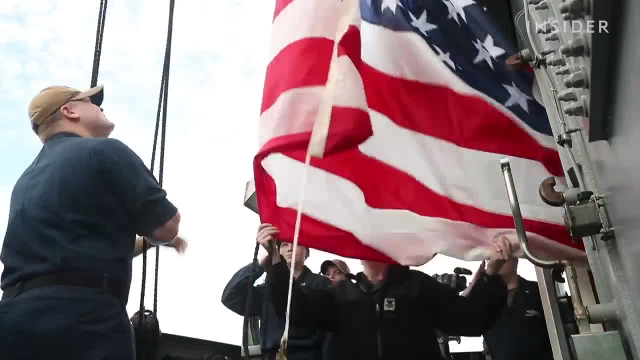 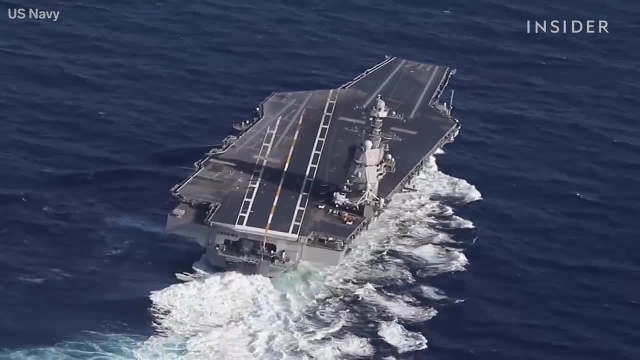 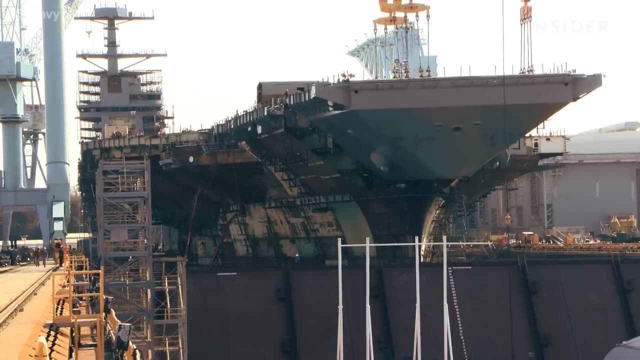 Navy, if you will. Of the 22 aircraft carriers in the world, half are American, while China, Italy and the UK have just two each. This carrier class- if we build 10 or 11 or 12, could go easily into the 22nd century. 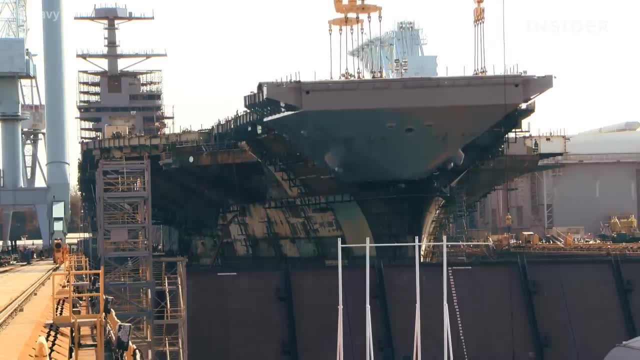 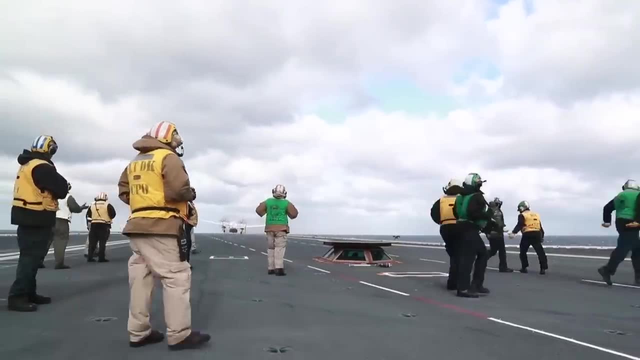 More than 5,000 shipbuilders worked an estimated 49 million hours to build the Ford. That's seven times the hours logged building the Empire State Building. Admiral Mike Gilday, the chief of naval operations, said it was a mistake to introduce more than 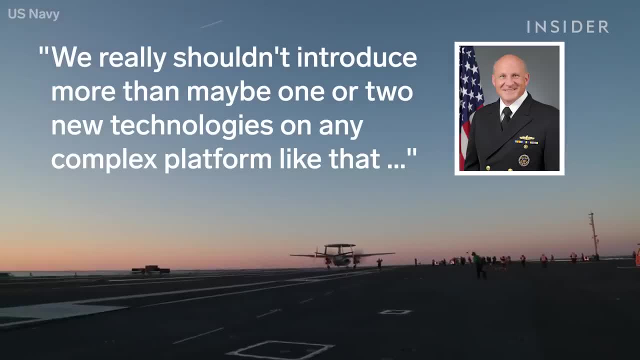 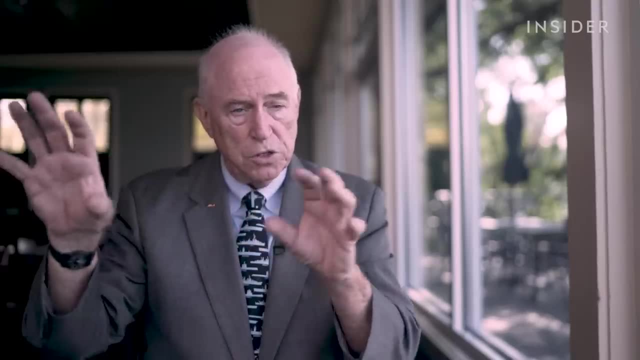 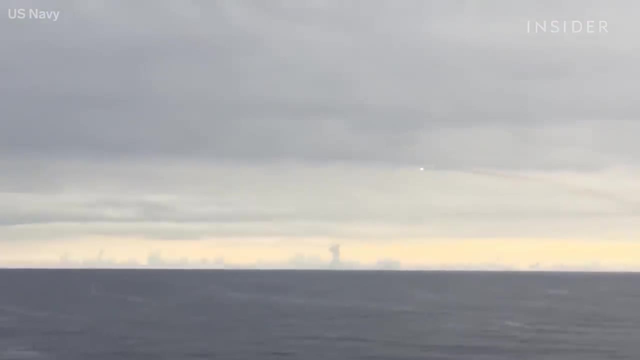 maybe one or two technologies on any complex platform at a time. Admiral Gilday is right: What you want to do is only do one or two new technologies on a new ship, And here's the reason why Ships are the only weapon that the prototype, the first of the class, goes to war on. 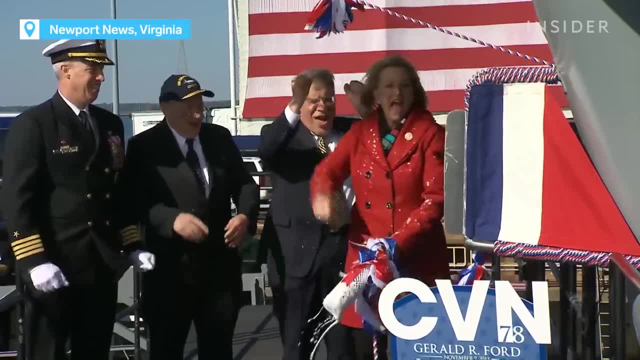 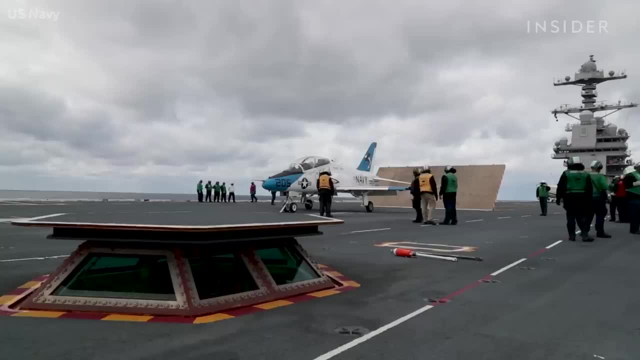 The ship was christened in 2013.. The Navy accepted delivery of the ship in 2017, without everything working, as a way to stay under that year's budget requirements. Four years later, the carrier's systems and technology are still being tested. And it won't be ready for deployment until 2022.. So it can go to sea, pilots can take off and land, but the problems are still being ironed out before it's ready to go to war. It's pretty clear that putting this many new technologies onto one ship was a mistake from 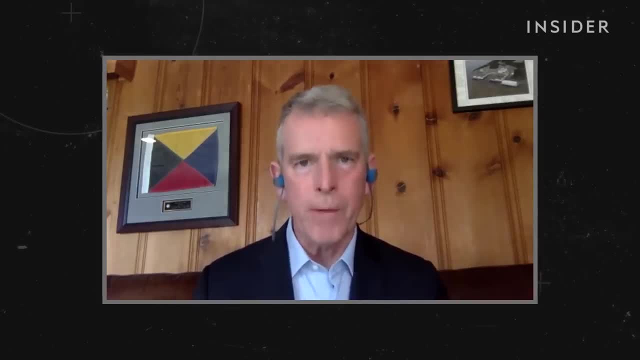 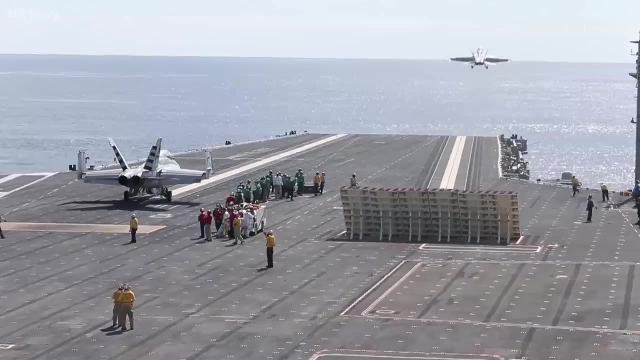 a program management perspective. Uh cause, it did cause a lot of trouble. It did cause the program to be delayed. The delays and tests and fixes are so costly that every new piece of technology is over budget. Two of the technologies that set the Ford apart from every other carrier are the aircraft. 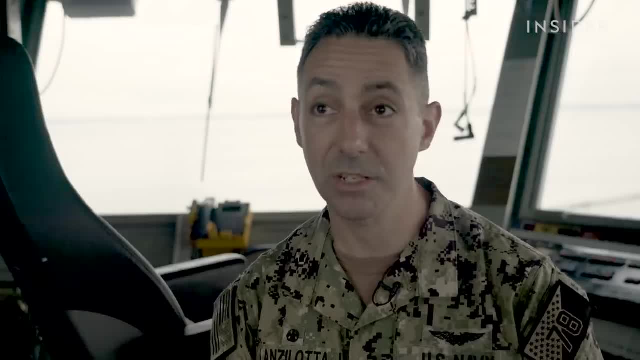 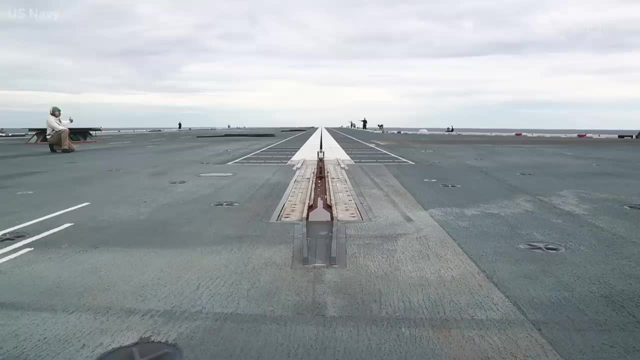 takeoff and landing systems. Some of those are very large, you know, not incremental changes, but I would say revolutionary changes in terms of the electromagnetic aircraft launch system. Other carriers use steam driven cabs. Some of those are very large. not incremental changes, but I would say revolutionary changes in terms of the electromagnetic aircraft launch system. 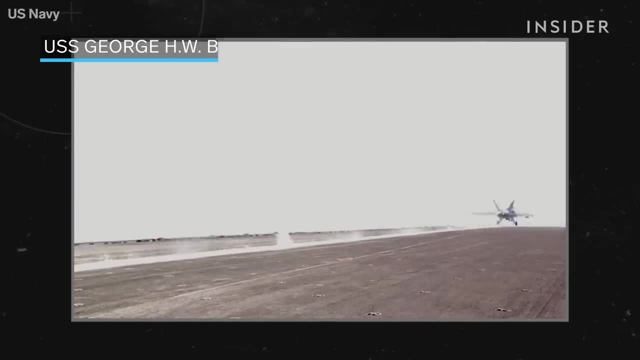 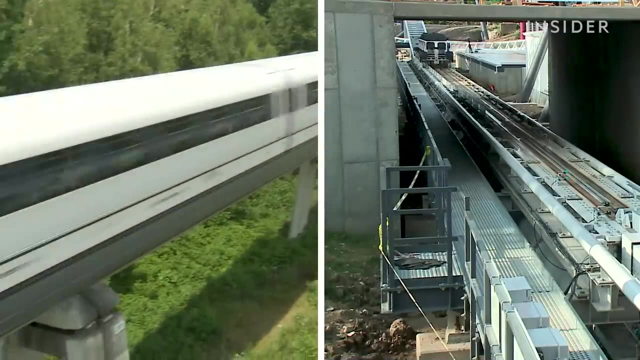 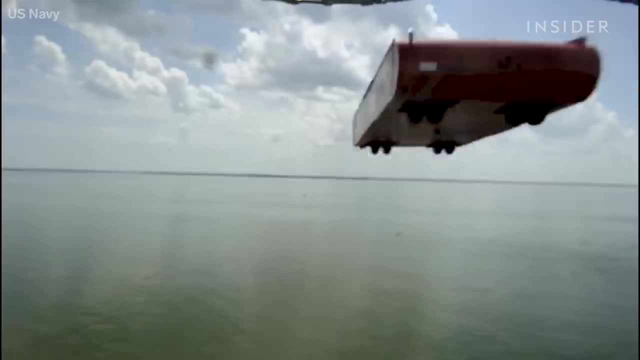 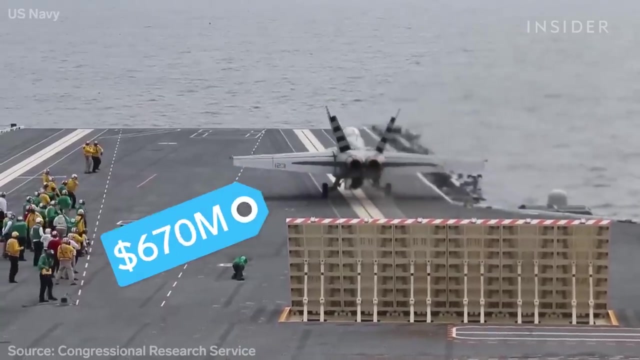 The Ford uses electric-magnetic linear induction motors similar to a high speed maglev train or roller coaster. Just research and design on the electromagnetic aircraft launch system cost over one billion dollars. Installing it on the USS Ford cost more than twice what it was supposed to. 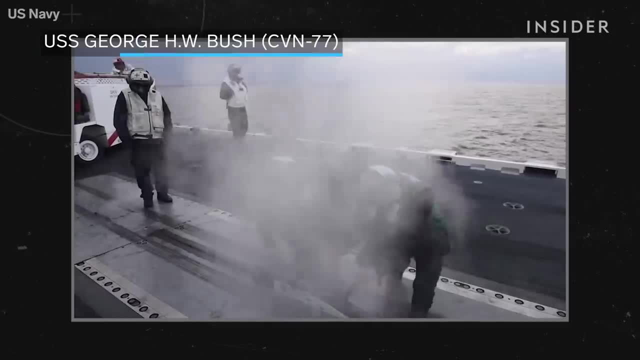 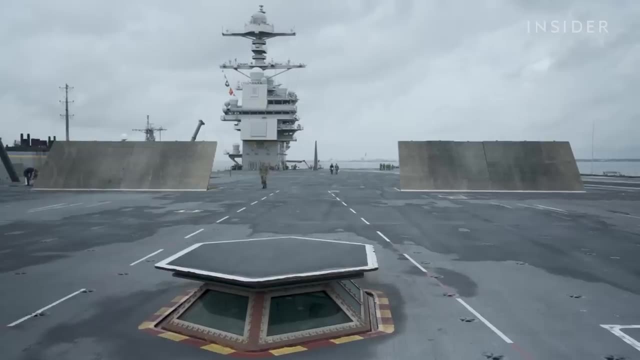 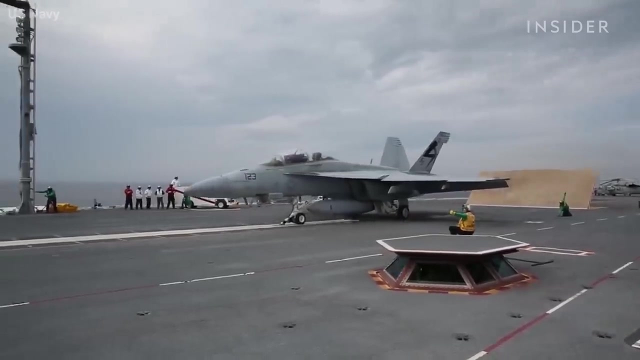 The steam catapult system had thousands of moving parts. It was a massive piece of metal. There are less than 100 moving parts on an electromagnetic catapult, so that was a big improvement. Fewer moving parts means fewer sailors to operate and maintain The smaller crew, and new technologies were projected to save $4 billion over its 50-year. 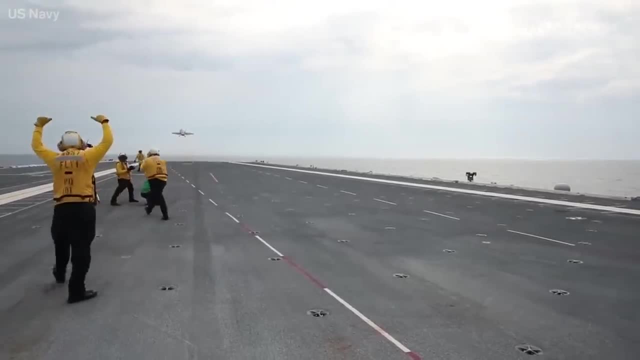 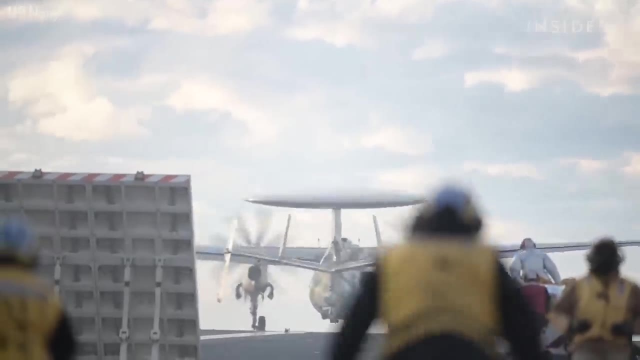 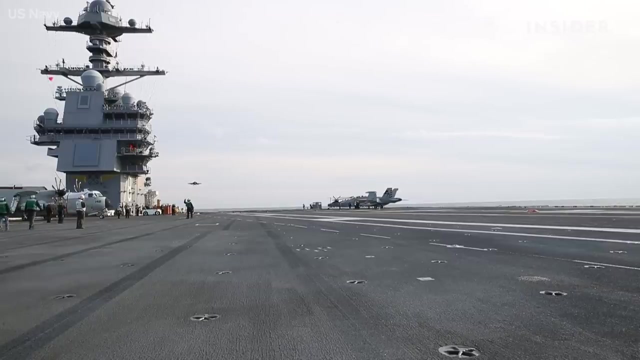 run. compared to the previous class of aircraft carriers, The new system causes less stress on the planes, so they last longer and more types of aircraft can use it, including ones that are still being designed. Landing and takeoff are easier on pilots too, since a computer does the work. 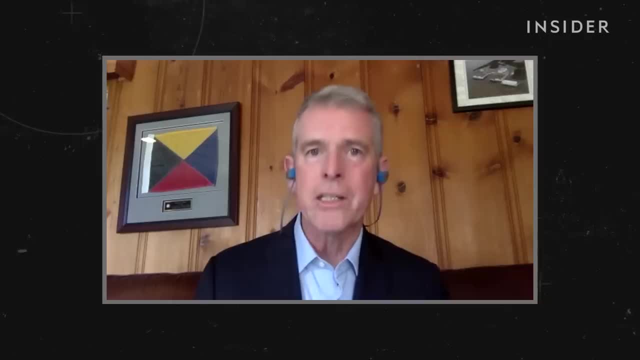 The pilot turns over control to the computer, It autopilots the airplane down to the carrier deck and then, when it hits that advanced arresting gear, it just smoothly brings it to a stop. So it's a dramatically different experience for the pilot. 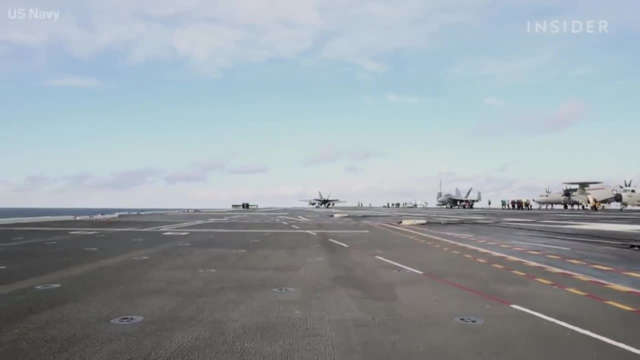 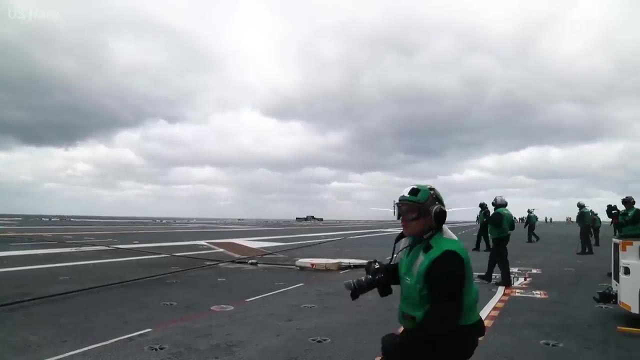 It's much safer, and then it's also going to make the airplane last longer. The Ford's computerized systems allow both life-saving and life-saving. It allows lighter and heavier planes to take off and land, something that limited older carriers. The Ford's combination of new technologies means that a wider variety of aircraft can. 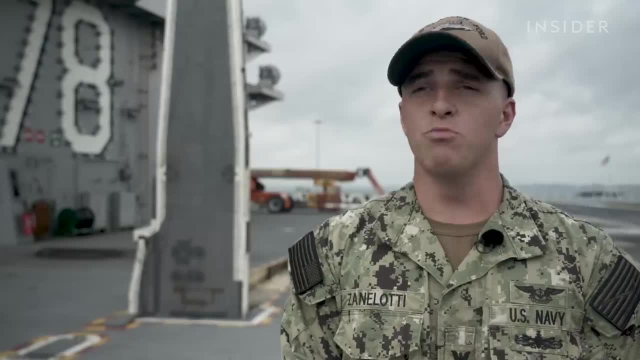 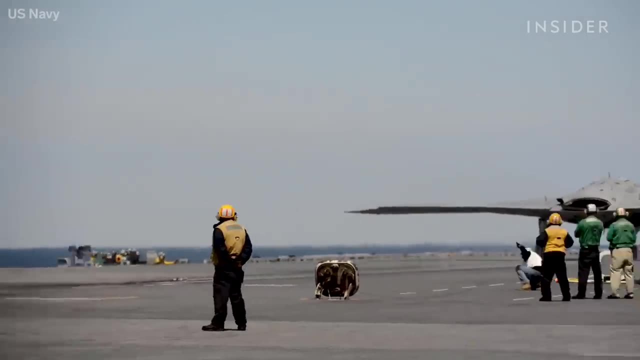 land on it. It's smoother arrestments for aircraft. That is our goal here on board for future of naval aviation flying drones and F-35s. Oddly enough, the new launch system can't handle the newest fighter plane, so the Ford. 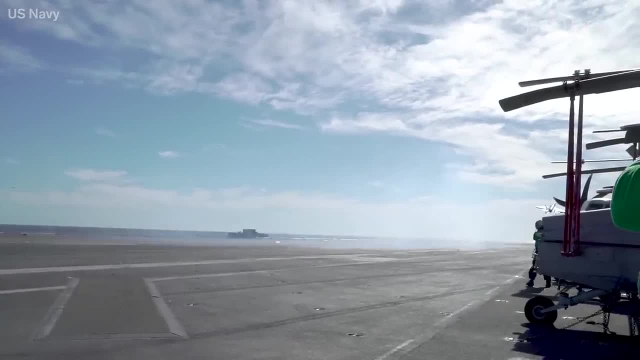 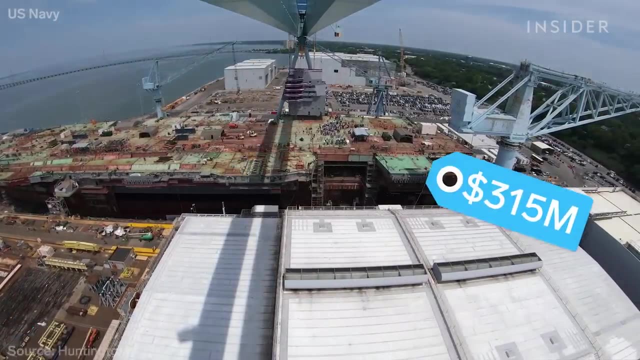 will need a retrofit to handle the F-35 stealth fighter. The next Ford-class carrier is the F-35.. The next Ford-class carrier is under construction in the shipyard, but it's already being modified for the F-35 at an added cost of $315 million. 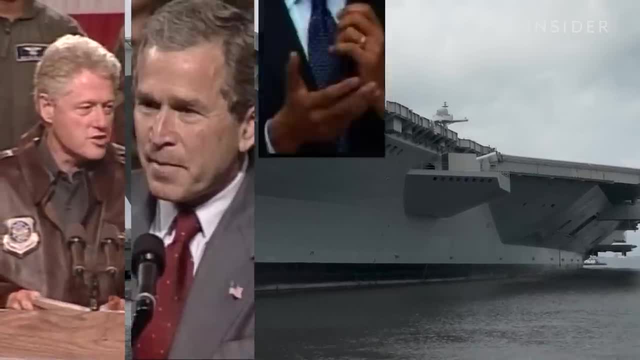 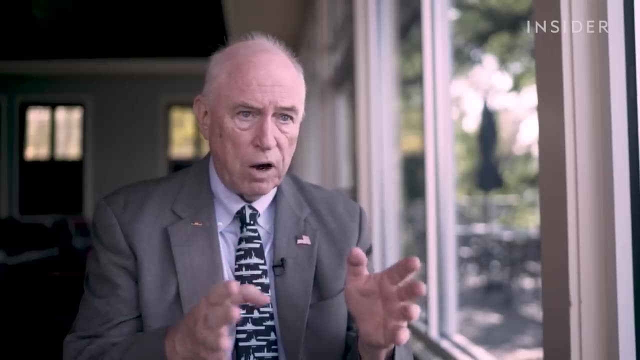 Many of the Ford's delays can be traced back to politics. Five American presidents over two decades weighed in on the planning and building of the Ford. The Department of Defense made the aircraft carrier program far more expensive than it needed to be, And you can take that to the bank. 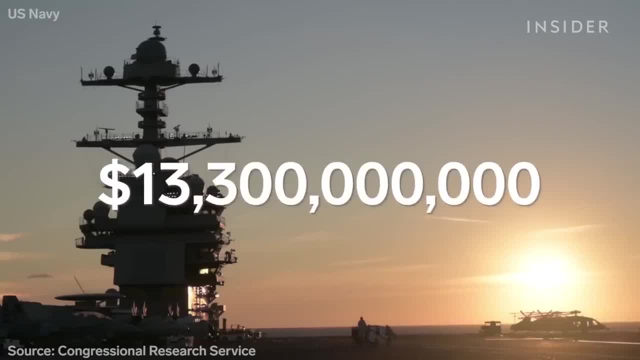 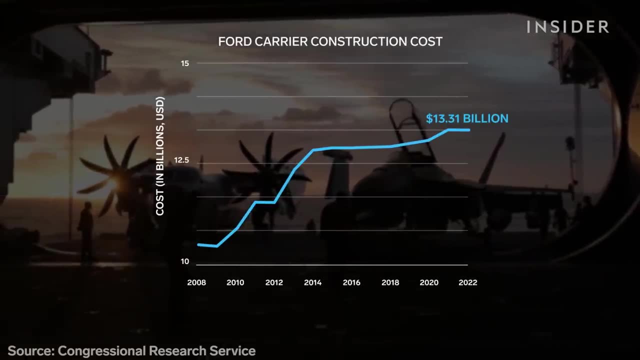 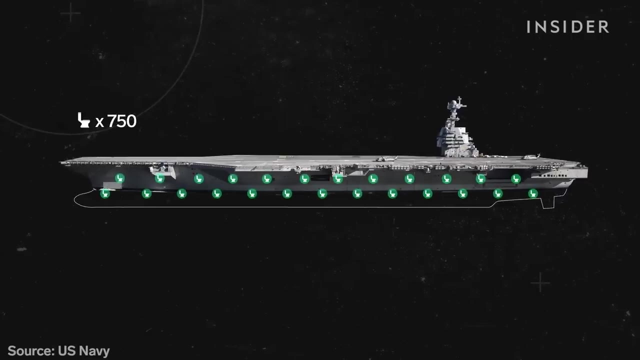 So far, the true cost of building this warhorse is $13.3 billion, a number that's increased nearly every year since construction began. Even the most basic of onboard functions can be eye-wateringly expensive. The ship has 750 toilets connected through vacuum pressure, like the system on commercial. 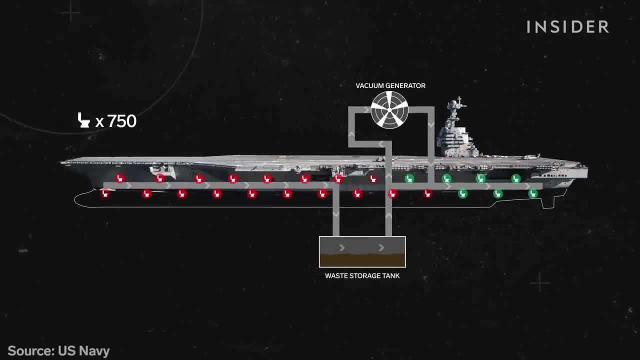 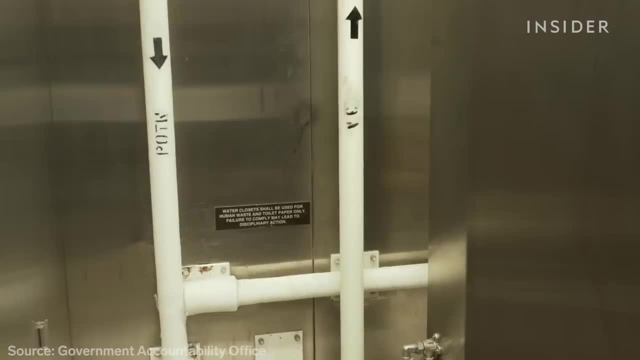 jets. When one toilet gets clogged, the whole system can be affected. The fix requires an acid flush that costs $400,000, and the Navy has said it doesn't know how often it will need to be done. The Navy changed its shipbuilding programs when the Ford's problems came up. 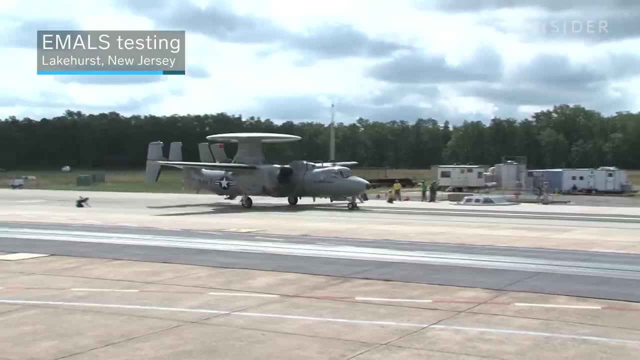 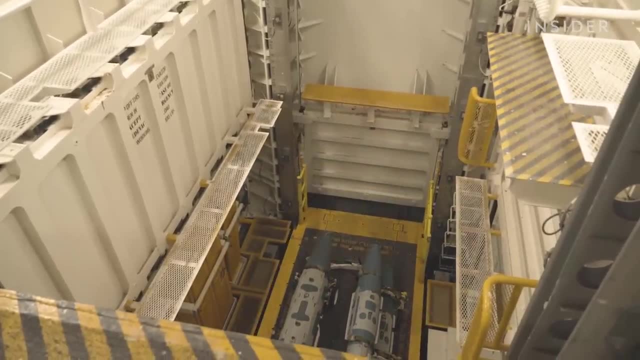 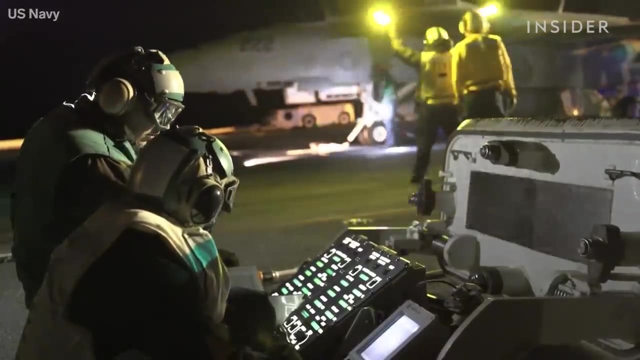 It began designing and testing the takeoff systems on land in 2011,, while the Ford was under construction. The advanced weapons elevators are also now being tested before installation. However, that program will only benefit the next Ford-class carrier. Built as a deterrent, the true value of the Ford is likely to be in the wars it helps. 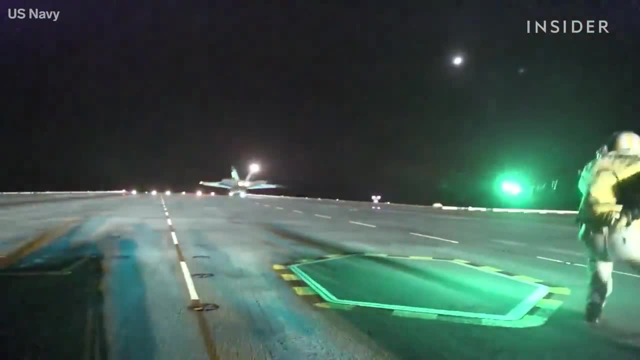 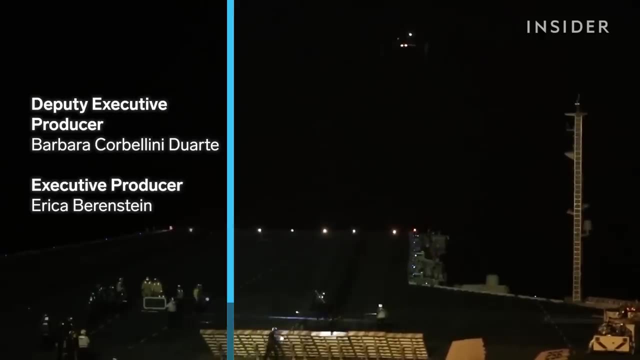 prevent rather than those it wages. The F-35 is the most expensive aircraft in the world. It vans up to $32,000.. In April 2019, the F-35 was the world's largest helicopter in terms of power and equipment.